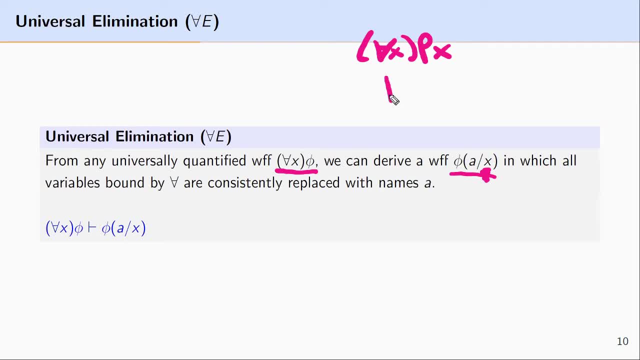 We would make use of universal elimination by removing the universal quantifier and replacing AXPX. We would make use of universal elimination by removing each instance of X with any name of our choosing, provided this replacement is uniform. So here we could replace the variable X, which is bound by the universal quantifier. here 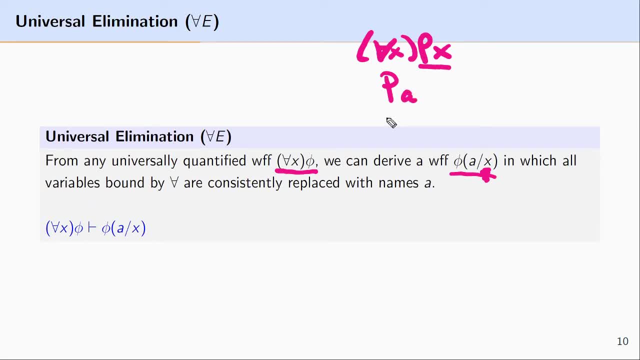 with, say, A, And we could apply universal elimination again and replace each instance of X with a different name, which is B. So again, the idea behind universal elimination is we reason from a universally quantified expression to a formula That the universal quantifier operates on, but we replace each bound variable X with 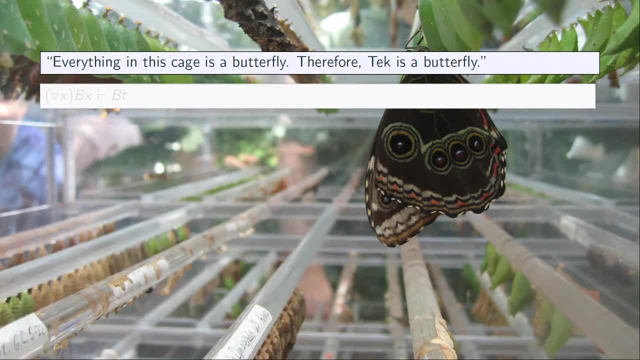 a name of our choosing. The idea behind universal elimination is pretty straightforward. It corresponds to how we reason using universal propositions. Someone might say: everything in this cage is a butterfly or is going to be a butterfly or in the future will be a butterfly. 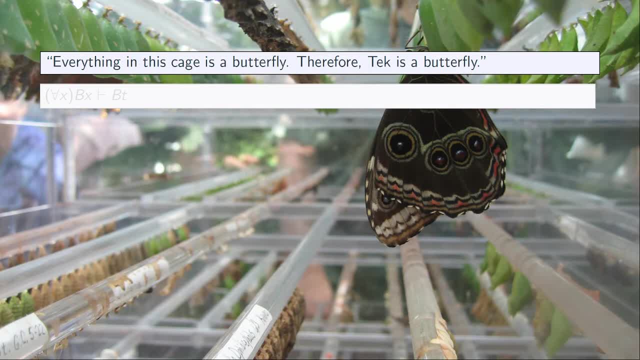 And from this we can reason to any specific item in the cage that we have a name for. so let's take a look at this particular butterfly that is very prominent in this slide and call this particular butterfly tech. So we can reason from everything in this cage is a butterfly to the statement tech is a. 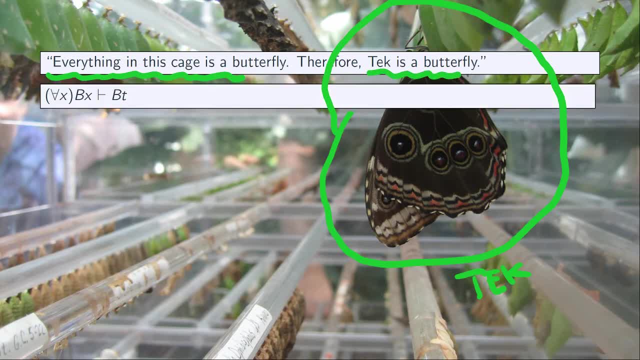 butterfly. We represent this in the language of predicate logic by saying: for all, X, BX, that is, everything in the domain of things that we're talking about is a butterfly. therefore, tech is a butterfly And what we've done Is simply to replace again, remove the universal quantifier and take the formula that the universal 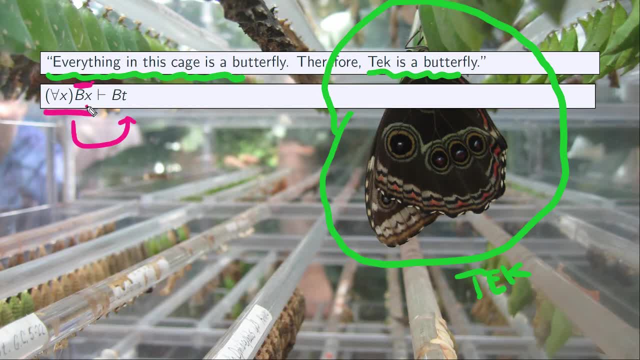 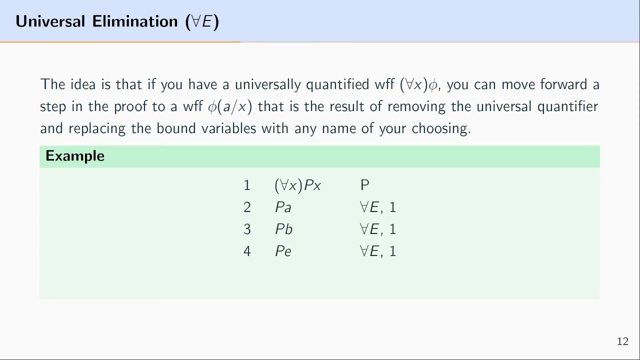 quantifier operates on and replace each bound variable with a name of our choosing, And in this case we picked T, because T refers to tech, here, this butterfly. Let's look at some further examples. The basic idea behind universal elimination is: you start with the universally quantified formula and 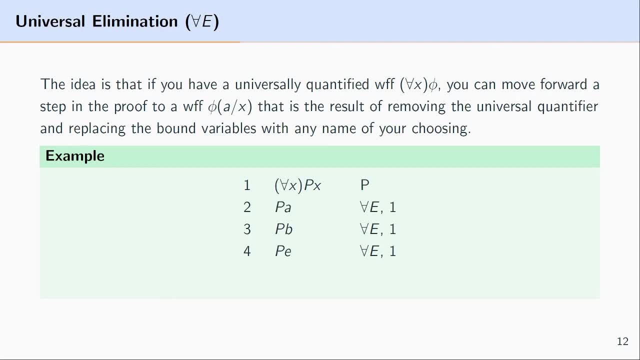 we, you can move forward a step in the proof. We've moved forward a step in the derivation by removing the universal quantifier and replacing the bound variables with any name of our choosing. So just to look at a quick example, here we have a X, P, X at line one and lines two, three and 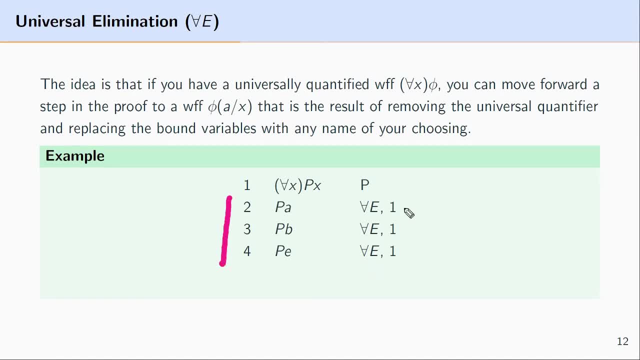 four are results of using universal elimination online One. at line two, we used universal elimination and replaced X with a. at line three, we use universal elimination online one. So we're reasoning from this universal quantifier Expression and we replaced the bound variable X with B. and at line four, we made use of universal. 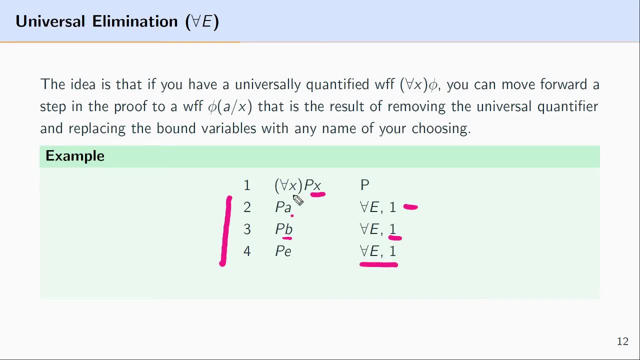 elimination, once again online. one replacing the bound variables X with E. So one thing to kind of note about this example is: the name we pick is completely up to us. And then, two, you can make use of universal elimination more than once on a particular. 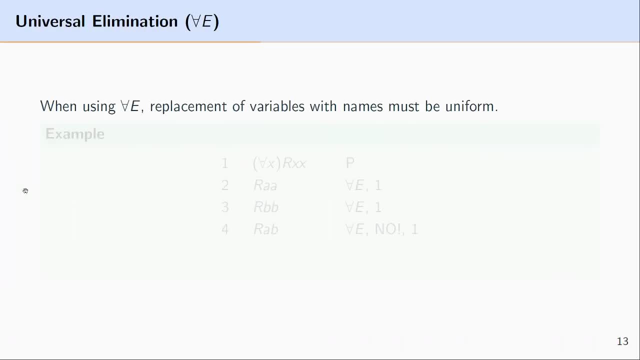 universally quantified formula. One mistake I sometimes see is that the replacement of variables with names- Okay Okay- Is not uniform. So the idea is that when you make use of universal elimination, this replacement of variables with name needs to be univ, uniform. 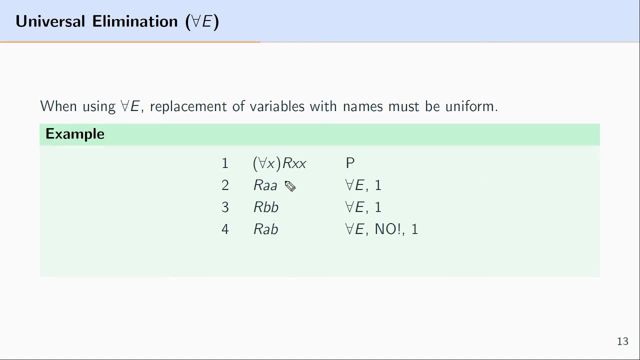 So let's look at an example of this here. at line one, we have for all X, R, X, X. at line two, we make use of universal elimination and we replaced all of the bound variables with a name, And that name is the same name. at line three, we have a use: 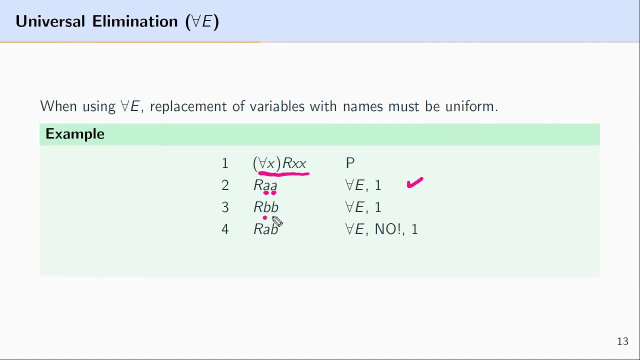 Of universal elimination, again online one, and we replaced the bound variables X with the same name. but line four is a case where we've taken those bound variables And in one case we replaced the X with a and the other case we replaced the X with B. 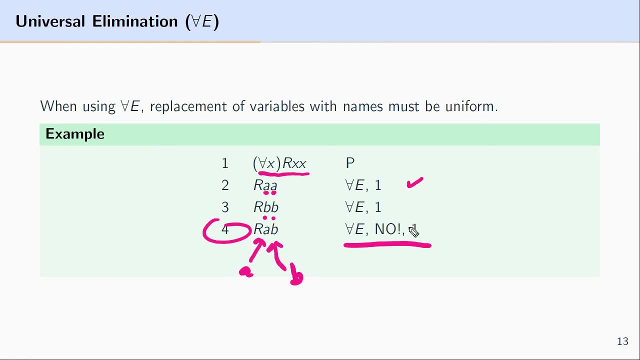 This is not a acceptable use of universal elimination. to see why: suppose line one says everyone loves themselves. So for any X in the domain That X is in the relation of loving themselves, it would follow that from line two, When we make use of universal elimination, we'd see that it would follow that Alfred loves himself. 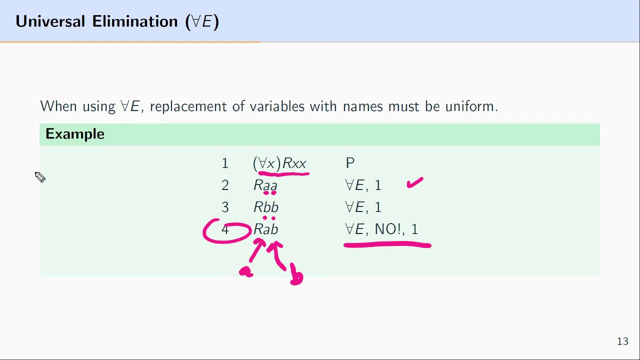 And this would seem to intuitively follow from line one: If everyone loves themselves, then Alfred loves himself. at line three We say that we have RBB and let's say B stands for Bob. This was line three- would say: Bob loves himself.